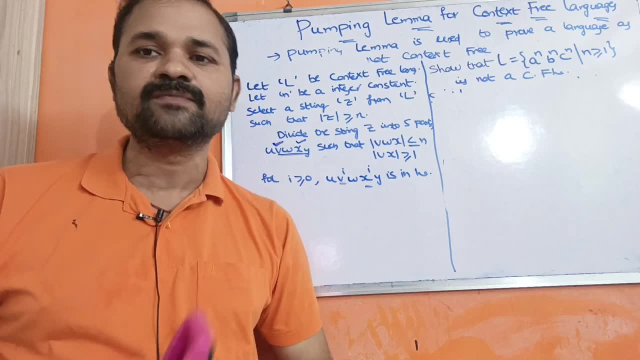 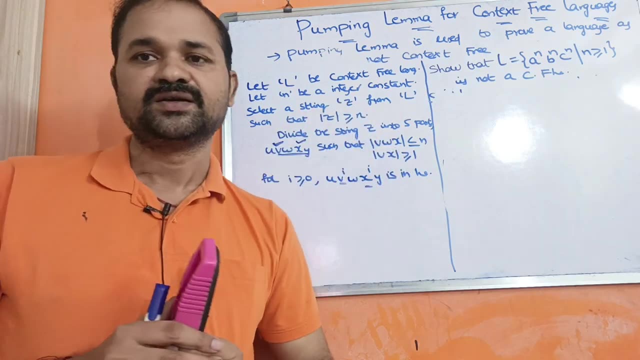 than or equal to N. So we have to select the string Z from the language L in such a way that length of that string is greater than or equal to N. Next, we have to assume the given language as context-free language. So we have to: 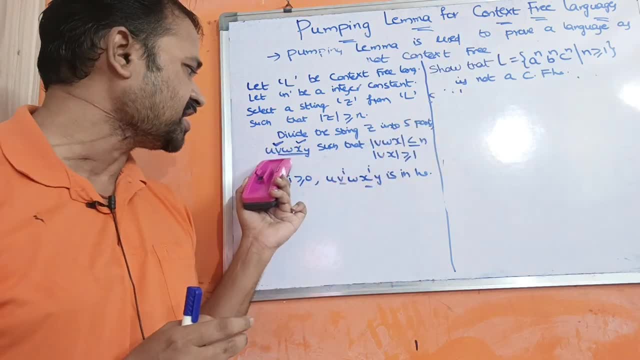 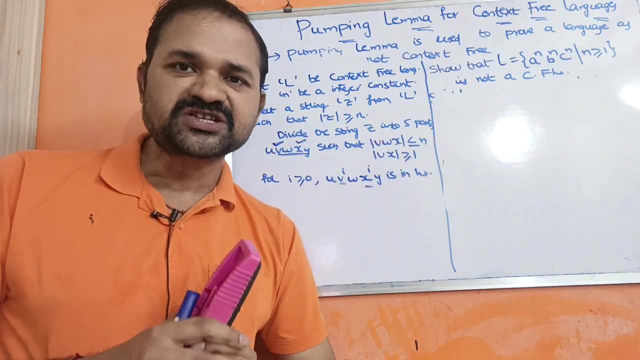 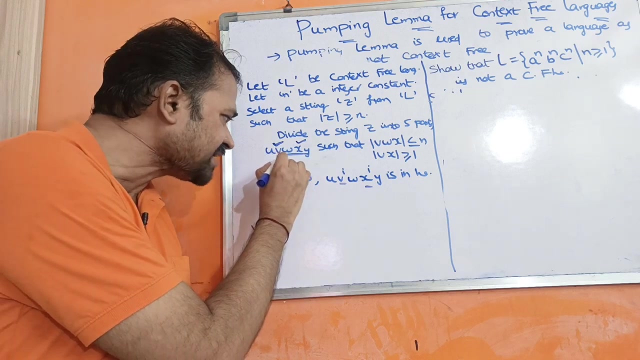 divide the string into five parts, such as U, V, W, X, Y, such that by satisfying these two conditions- The first condition is: mod VWX is less than or equal to N. Here VWX is nothing but middle part. So this middle part should be less than or equal to N And the 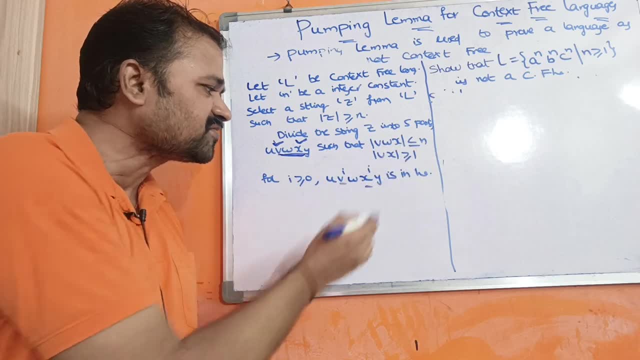 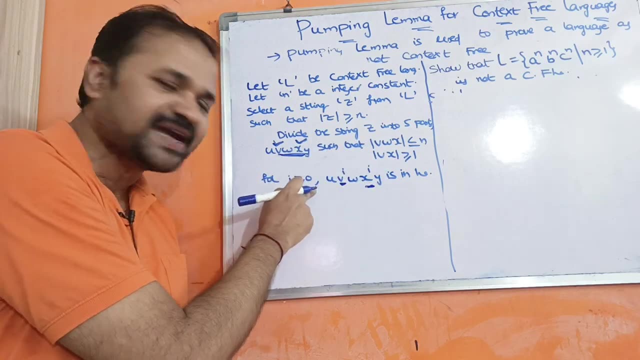 second condition is: mod VX is greater than or equal to 1.. Why? Because here we have pump in, We are incrementing V and X value. Initially I value is 0.. Next I value is 1.. Next I. 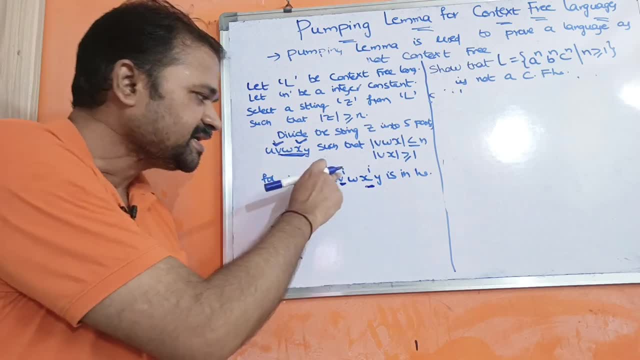 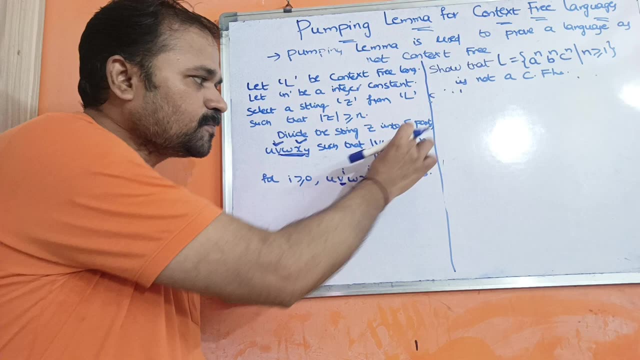 value is 2.. So pumping means incrementing. Here we are incrementing V and X. So that's why the condition is: mod VX is greater than or equal to 1.. So by satisfying these two conditions we have to divide the string into five parts, If these two conditions are. 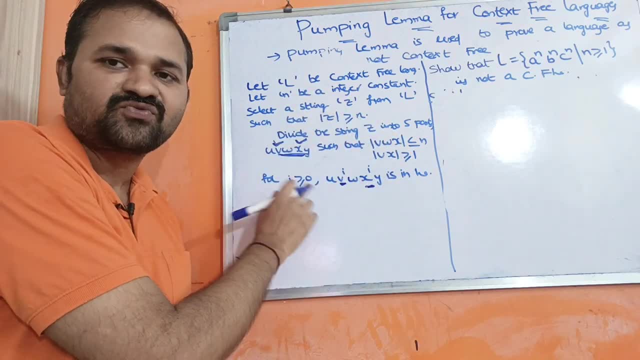 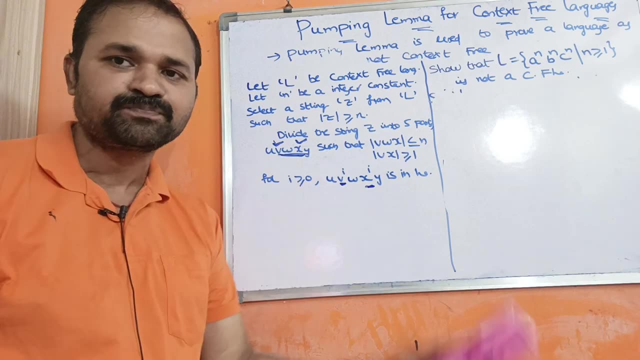 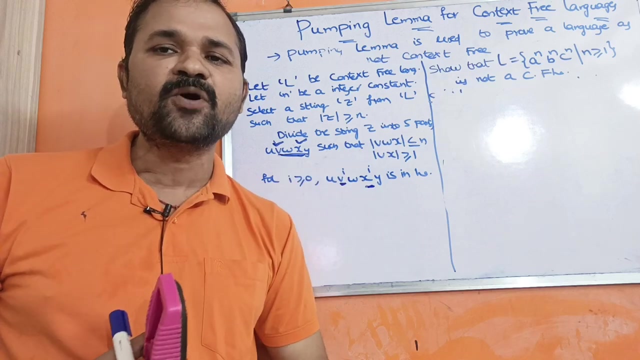 satisfied, then we have to check this condition also, For I is greater than or equal to 0,. u v power i, w, x, power i, y is in l. okay, so this is the theory here. now let us solve the problem. show that l is equal to a power n, b power n, c, power n, such that n greater than or equal to 1. 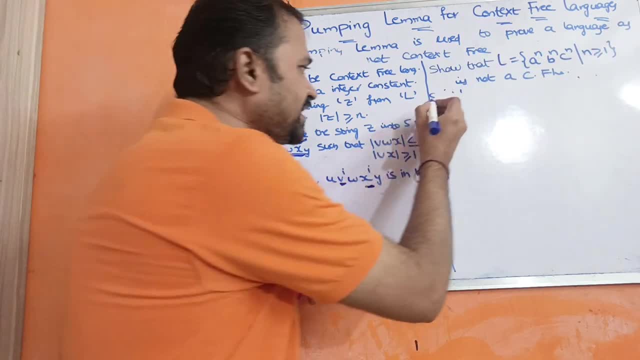 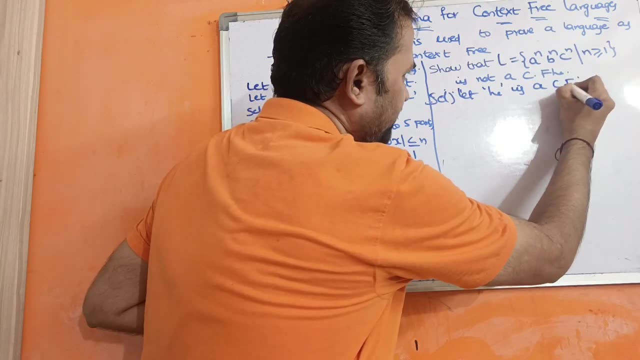 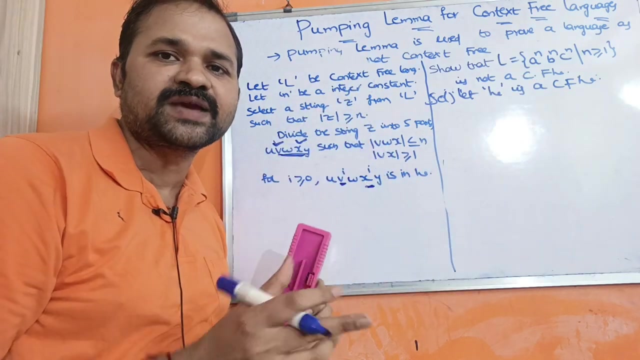 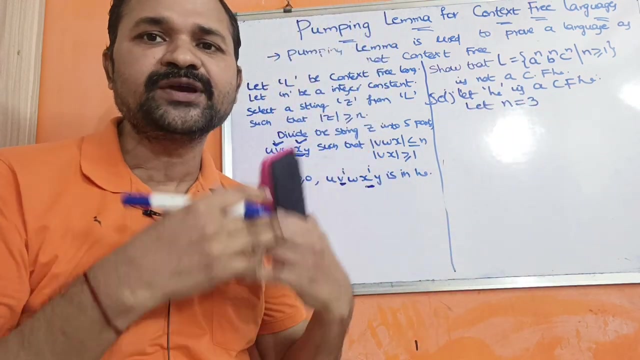 is not a context-free language. so let us see the solution. initially, we have to issue this language as the context-free language. let l is a context-free language. next, we need to assume an integer value. let n is equal to 2 or n is equal to 3. it is our choice. we have to assume. 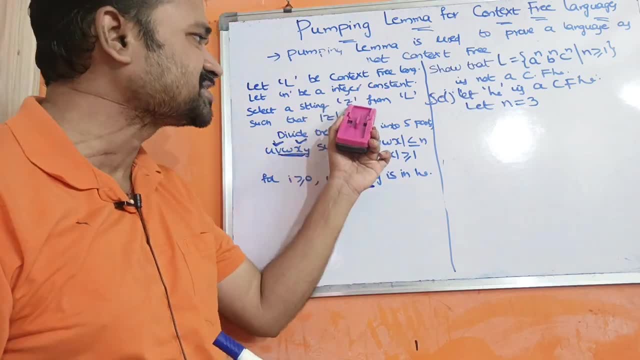 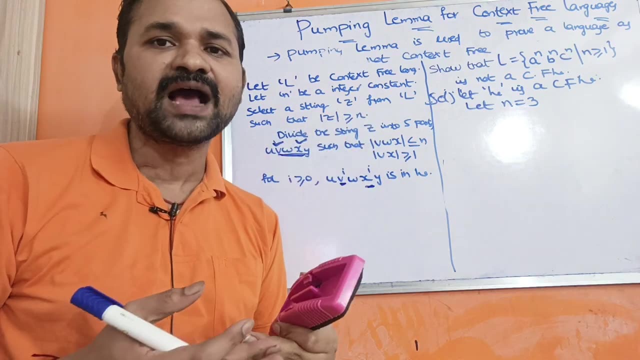 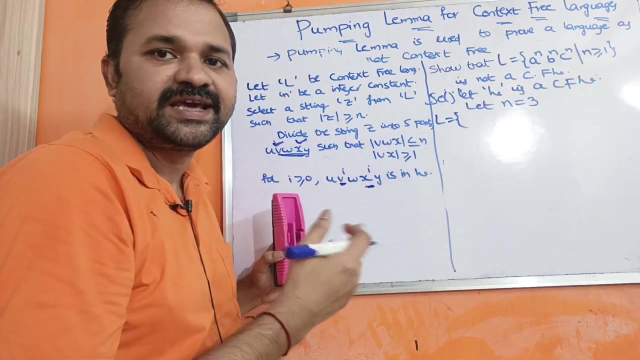 one integer value and we need to select a string, z, from the language n, such that more z is greater than or equal to n. so first we have to write the language. so l is equal to n, to suppose here n value starts from 1. if n is equal to 1, then what is the string? a power 1 is. 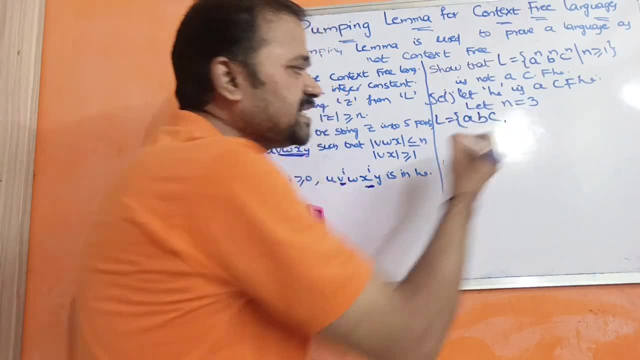 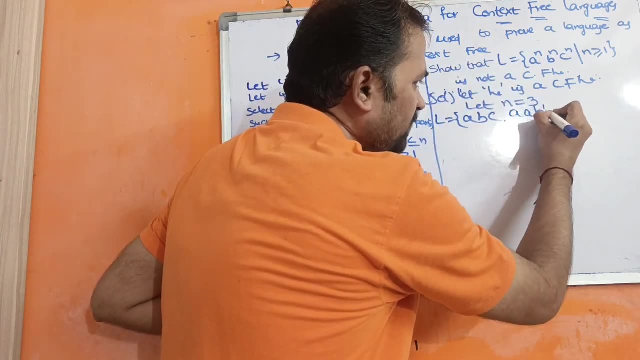 nothing but a, b. power 1 is nothing but b, c. power 1 is nothing but c. suppose if n is equal to 2, then a power 2 means a, a, b. power 2 means b, b, c. power 2 means c, c. if n is equal to 3, then a power. 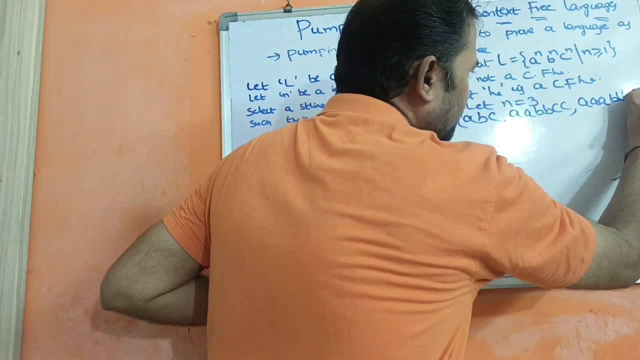 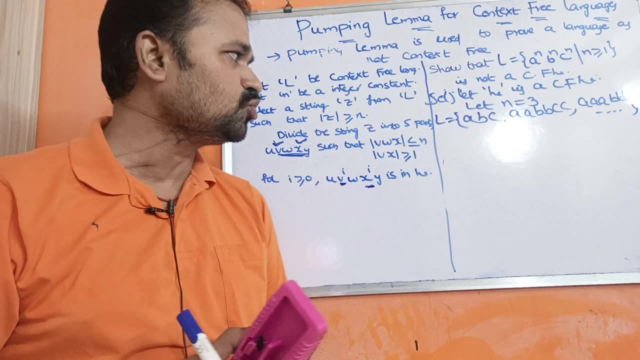 3 means 3. a's b power 3 means 3 will be c. power 3 means 3 will see so so on. so likewise, we can have n number of strings. now we have to select a string here. we are assuming that n is equal to 3. 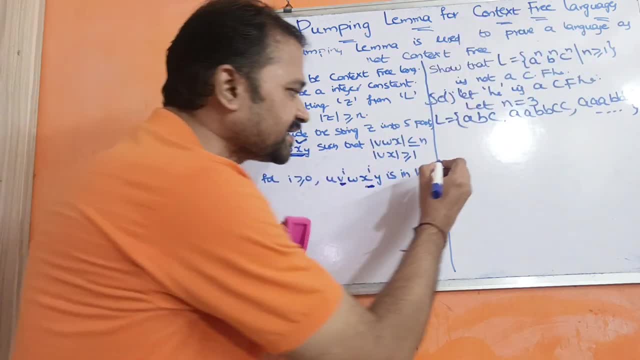 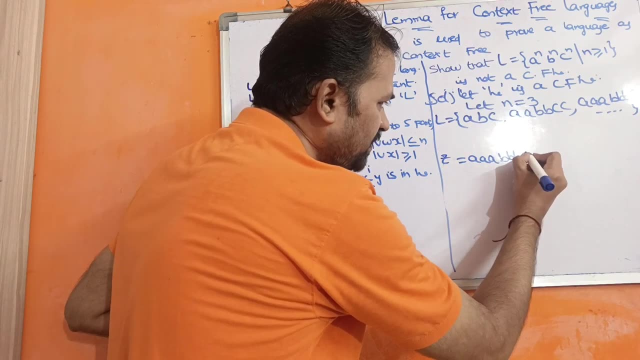 if n is equal to 3, then what is the string we will get that is equal to what is the string: a power a. power 3 means 3. b power 3 means 3 will be. c power 3 means c will see, 3 will see. 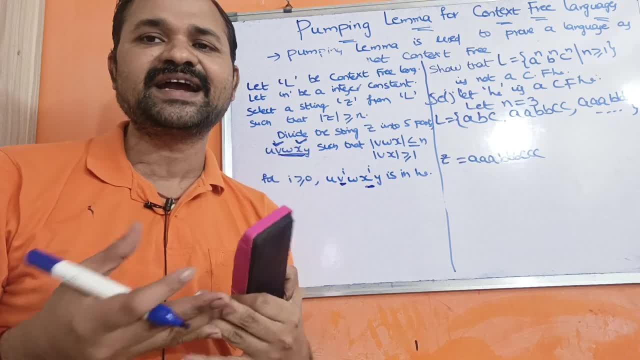 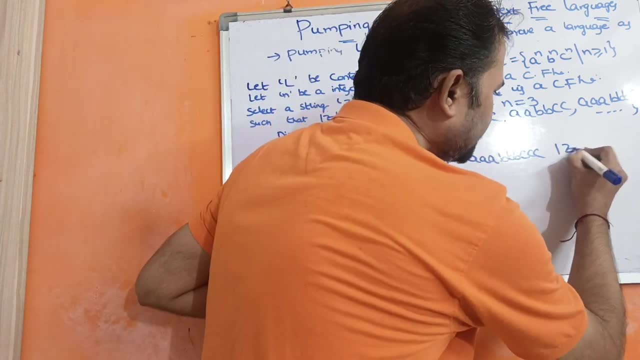 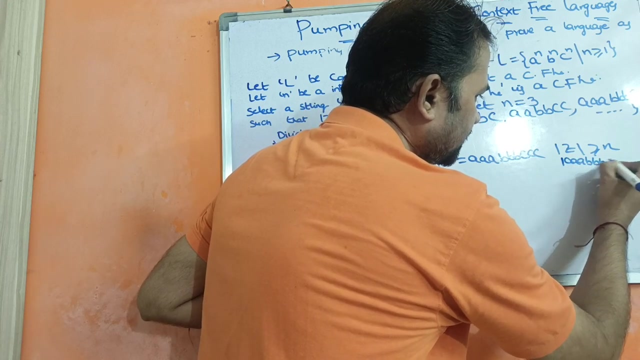 now we have to satisfies that condition, whether that condition is true or not. if this condition is true, then only we can select the string. so what is the condition? mod z is greater than or equal to n. what is mod z here? mod triple a, triple b, triple c is greater than or equal to what is n? value 3. so what is the 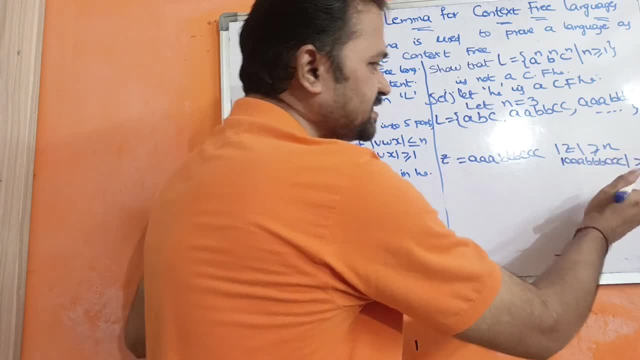 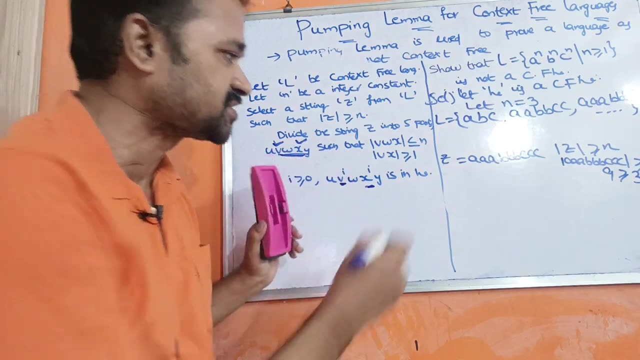 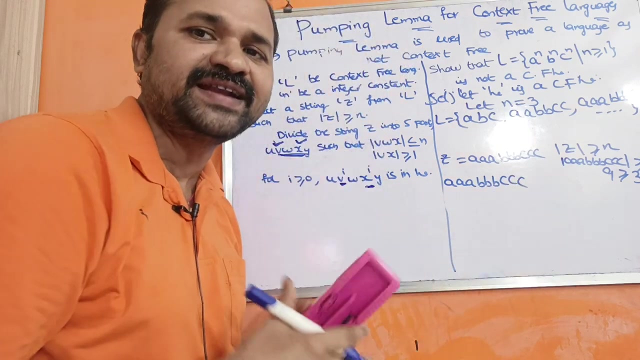 length of triple a, triple b, triple c, 3 plus 3 plus 3, 9. so 9 is greater than or equal to 3. condition is true. so we can divide the string into five parts. so what is the string? triple a, triple b, triple c. so we have to divide this thing into. we have to divide this thing into how many. 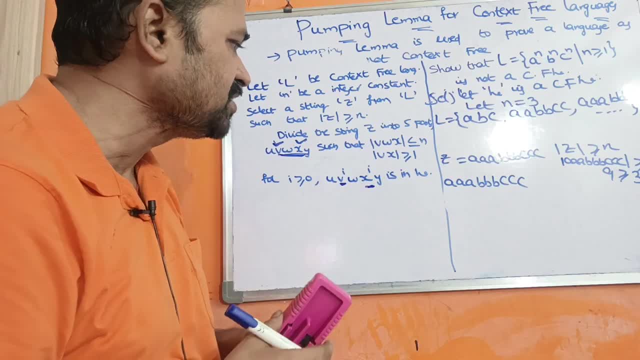 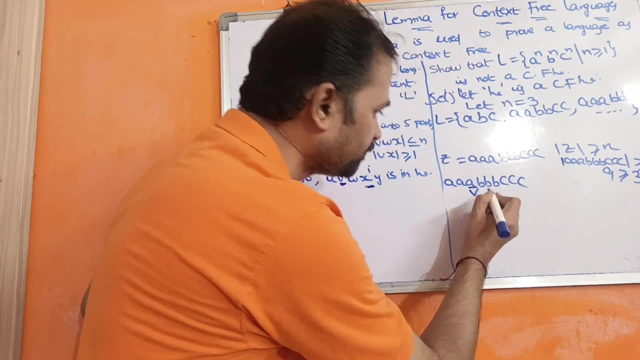 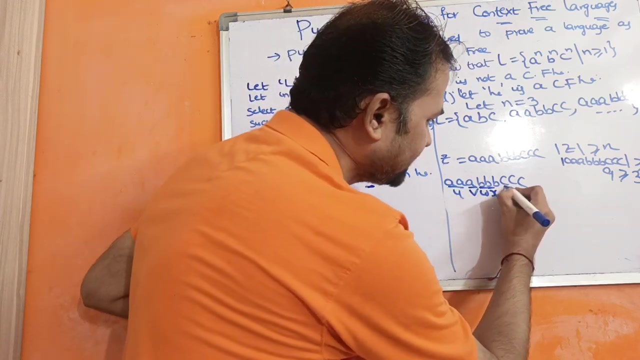 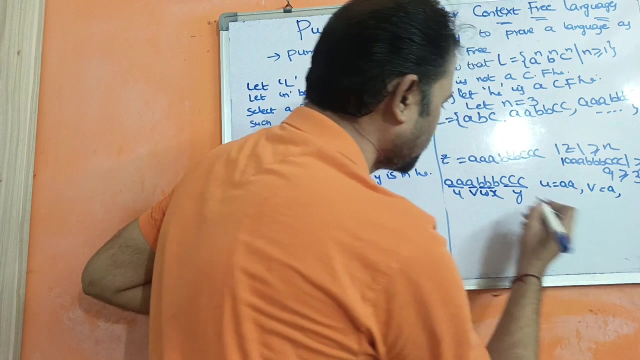 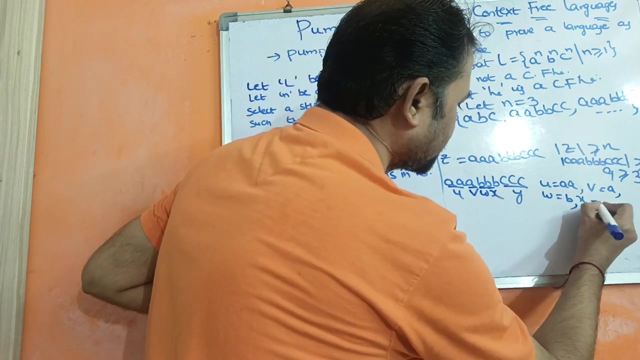 parts. uh, five parts. okay, uv, w, x, y. so here we have two conditions, are there? let us assume that this is v, this is w, this is x, this is e, is U and this is Y. so U means double, A, B means A, W means B, X means B, whereas Y means. 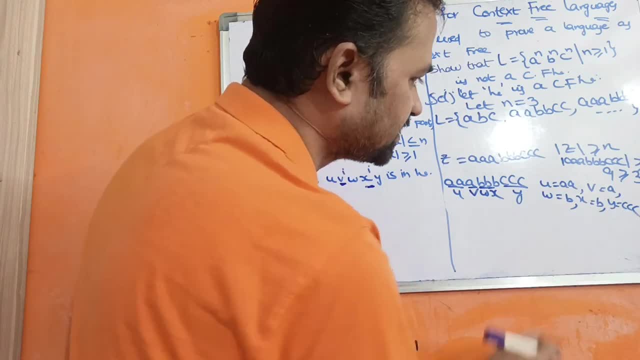 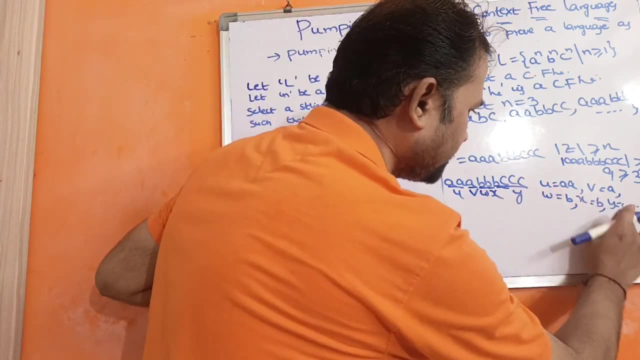 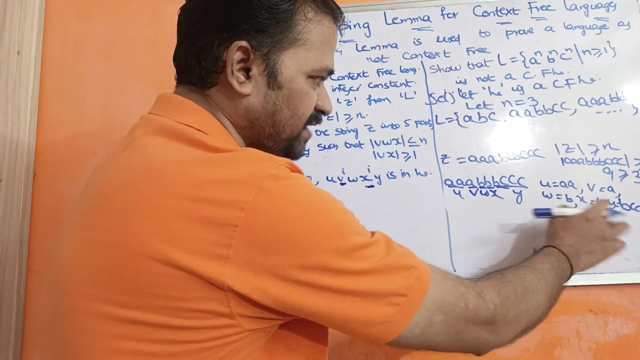 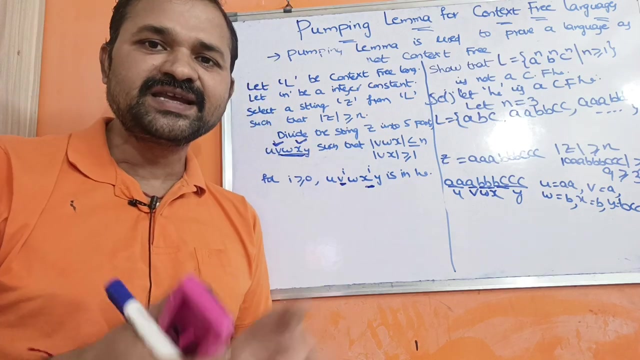 triple C, so triple A is over, next triple B, so one B is left. U, V- let us assume that this is W, so Y, triple C, B. triple C, B, triple C, so U, V, W, X, Y. okay, U, V, W, X, Y. U means double A. triple A is over, next. triple V is over, triple C is over. we can assume in any order, but we 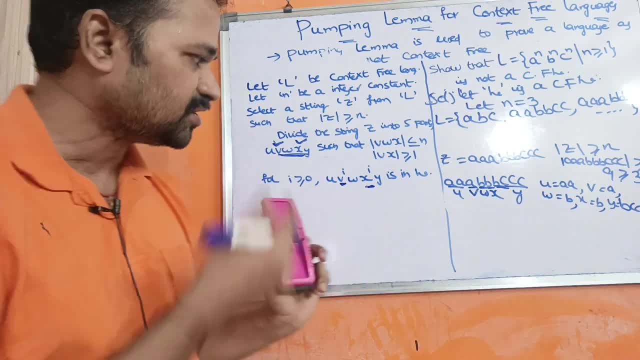 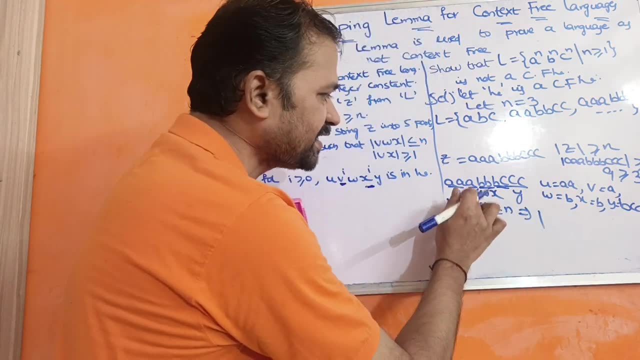 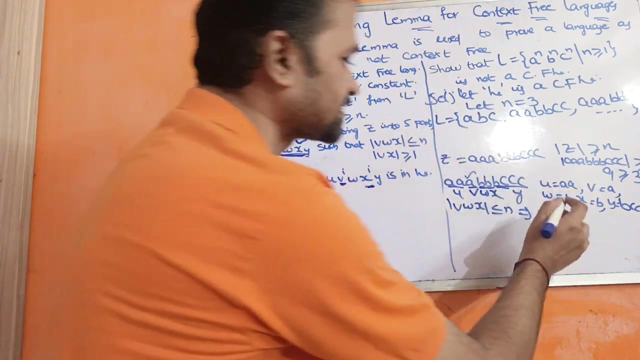 need to satisfy those three conditions, those two conditions. what is the first condition? mod V, W, X is less than or equal to N. mod. what is V here? V means A. what is W, B? what is X, V, W X? X means B is less than or equal to N. less than or equal. 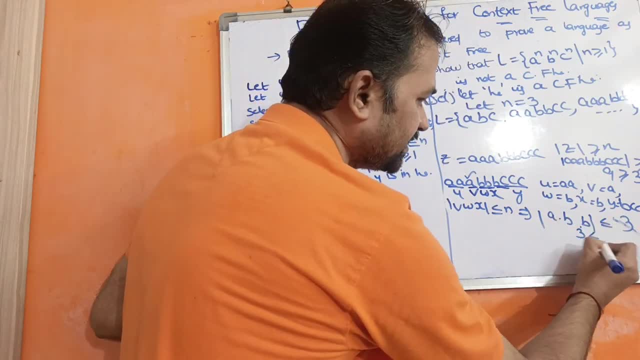 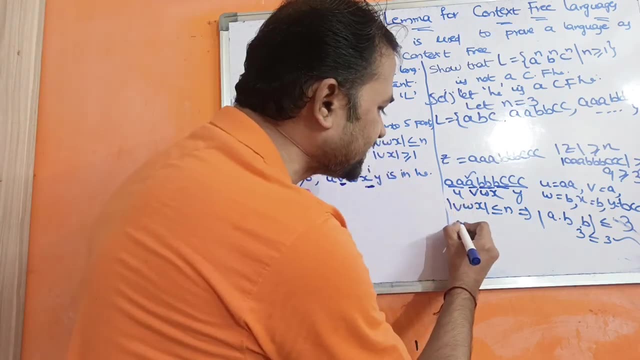 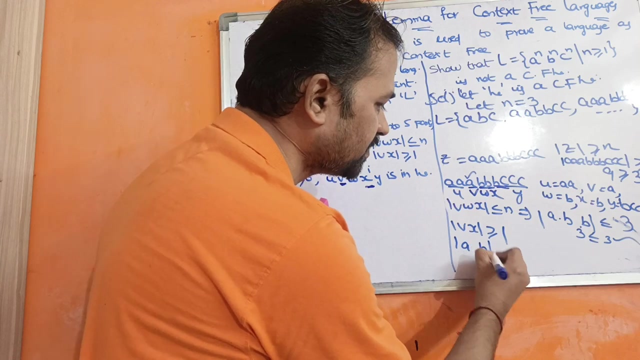 to what is N, 3. so what is the length here? 3, only 3 less than or equal to 3 condition is true. let us take the second condition. what is the second condition? mod V X is greater than or equal to 1. mod V X is greater than or equal to N. what is V A? what is X B? what? 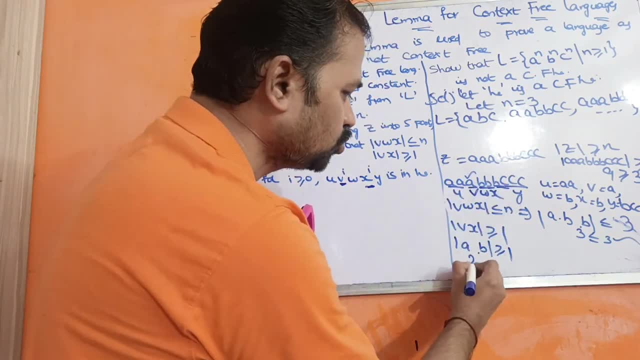 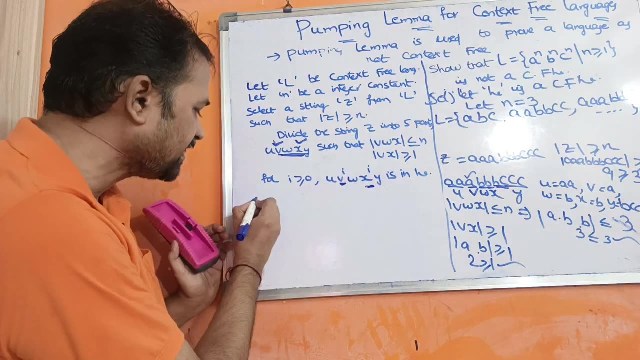 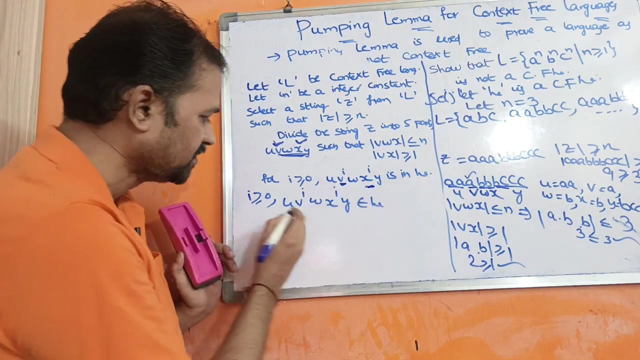 is the length of A, B. B means A, X means B. 2. 2 is greater than or equal to 1. condition is satisfied. now we have to check this condition for space constraints. I am writing here for I greater than or equal to 0. U, V, power, I, W, X, power I. Y belongs to N. let I is equal to 0. what is U value? what? 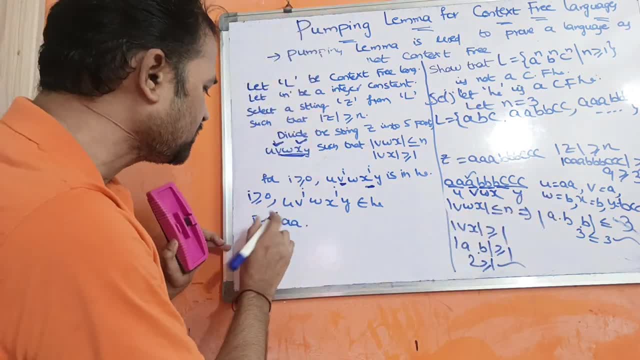 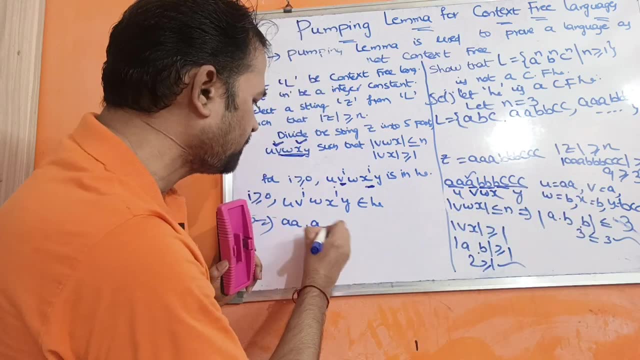 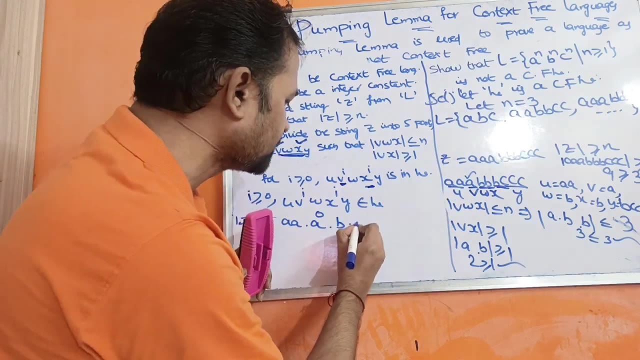 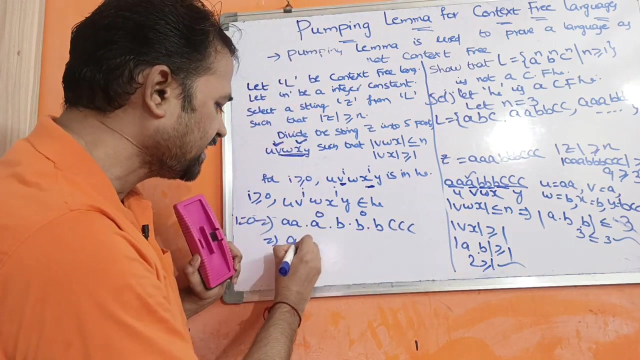 is U value double A. what is V value? for I is equal to 0. what is V value? what is V value? take name Este, catch 0, then this is V A power. here we are assuming ia 0, W means B, X means B, V power 0. what is Y? Y means B triple C, so A into A power. 0 means epsilon, epsilon. 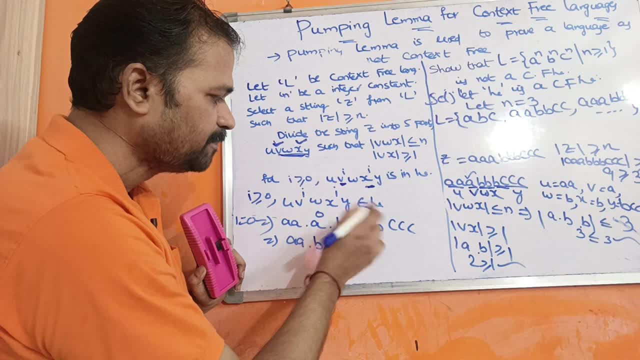 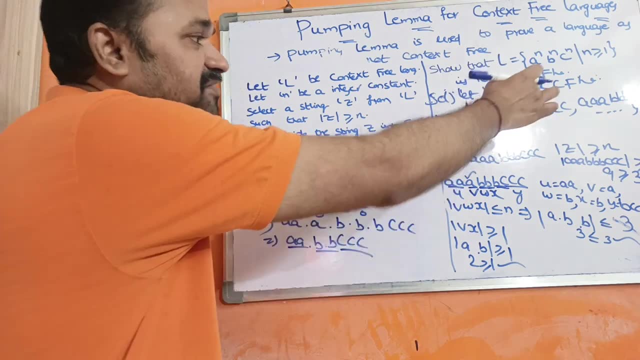 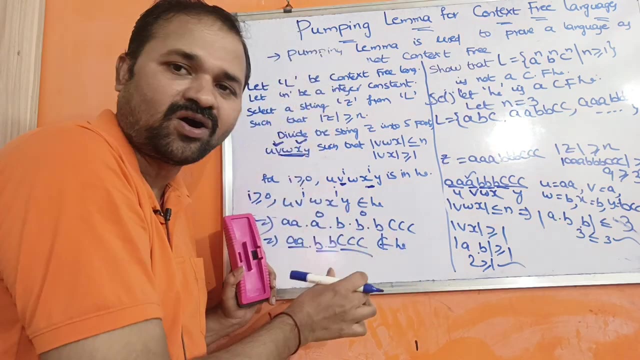 into anything is nothing but that, anything B into V. power 0 means epsilon, so V B, triple C. ok, here we got double A, double B, double C, but this line was: but this thing is not present in the line base, so this string is not present in the language. so we can, here we got the contradiction, is it? 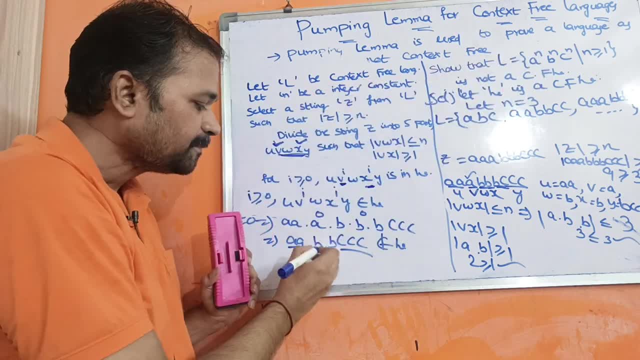 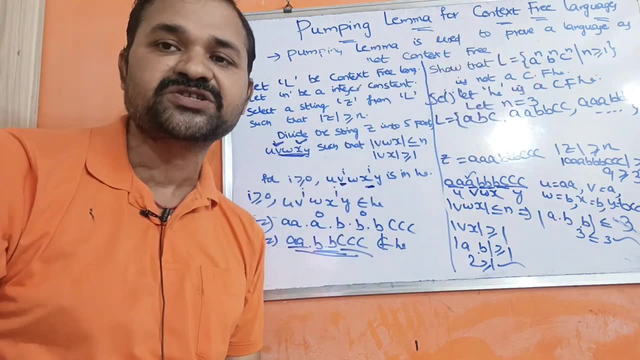 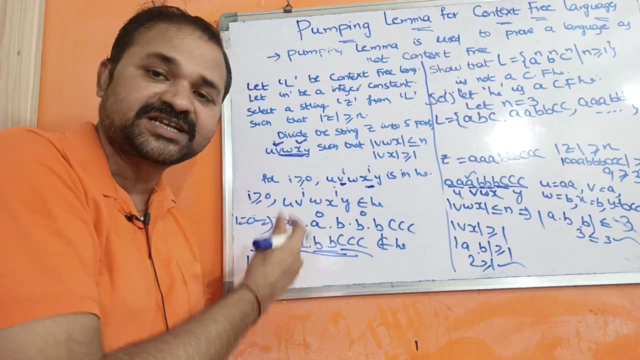 initially we assumed IAS- context-free language. but here we got a string which is not present in the context-free language, so we can say that our language is not context-free. suppose if this string is present in the language, then we have to assume IAS 1 and generate the next string. 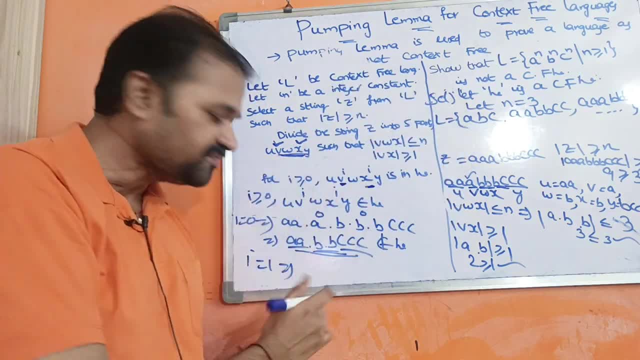 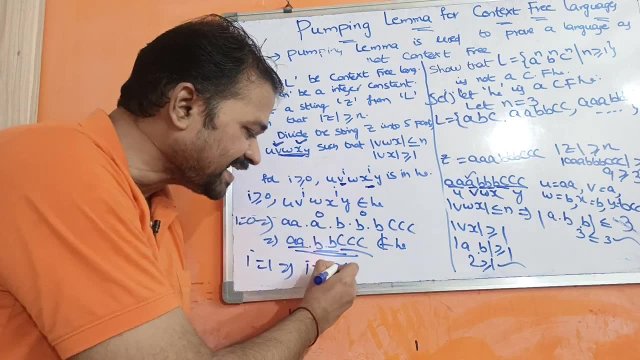 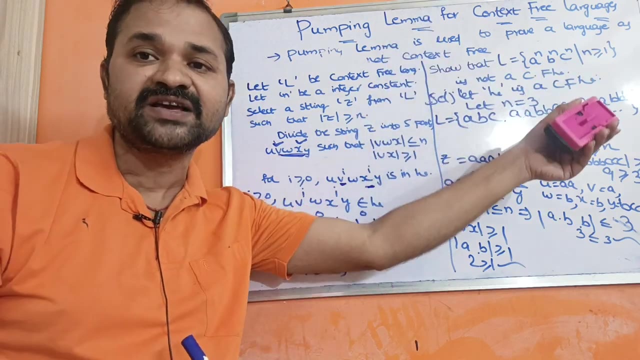 suppose if this string is also present in the language, then we have to issue IAS 2 and generate a string. so, likewise, we have to generate the strings until we get a string which is present in the language. if that string is not present in the language, then we can say that this language 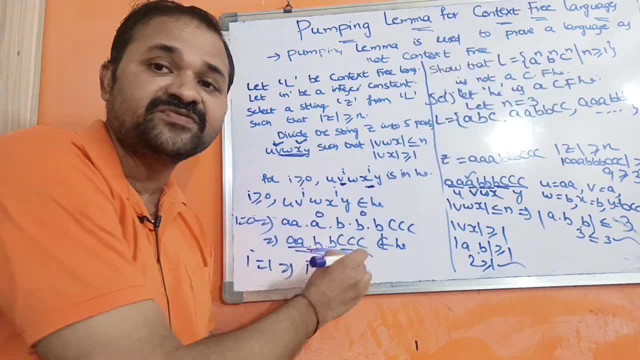 is not context-free. here we got a string which is not present in the language, so we can say that this is not context-free. you, you. 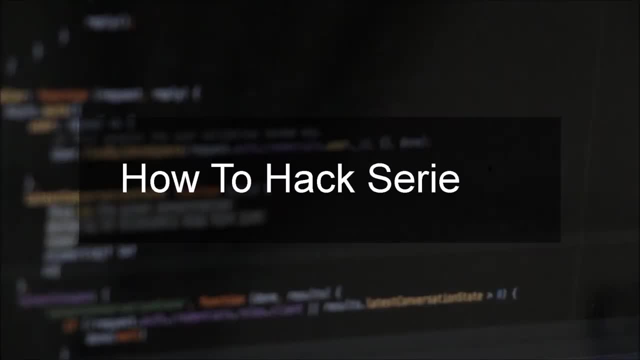 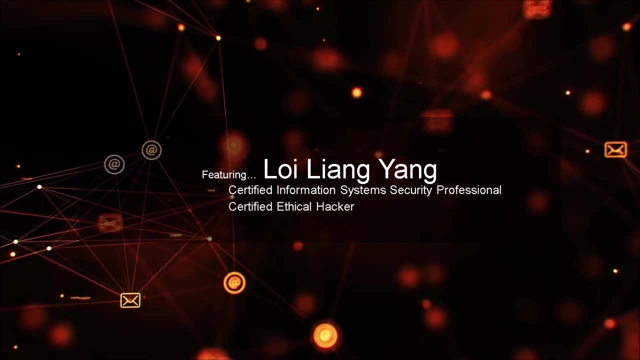 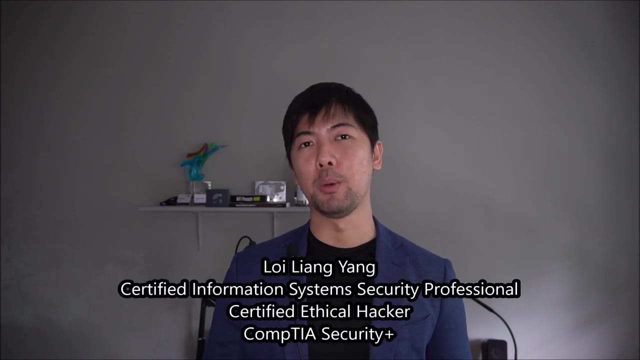 Hi and welcome back to another episode on how to hack. So today we're playing defense again, and what we'll be doing is installing Snort, which is an intrusion detection system that is host based and you can install it on your Windows operating system, and what it does is that it 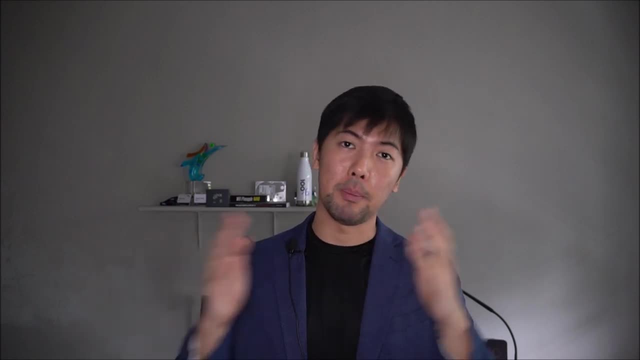 will intercept all the packets of TCP IP traffic that's coming in and out of the operating system and from there you can actually put in some of the advanced rules to actually see whether there are indicators of compromise, indicators of attacks, and directly from there you'll be able to do a lot of processing and rule based engine classification to see what. 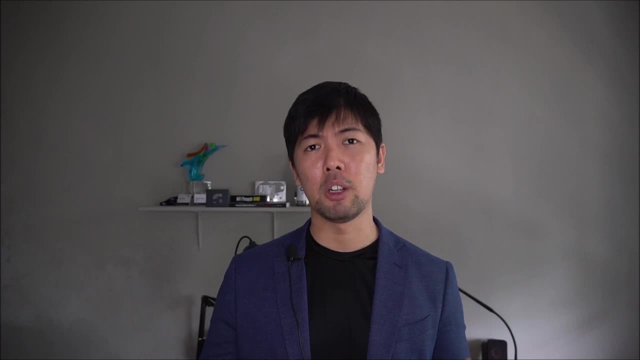 kind of attacks is going on. So it's a fantastic way for you to install, set up an intrusion detection system in each of your server or machine and be able to detect and flag up potential threats. So, without further ado, let us get started on today's tutorial. 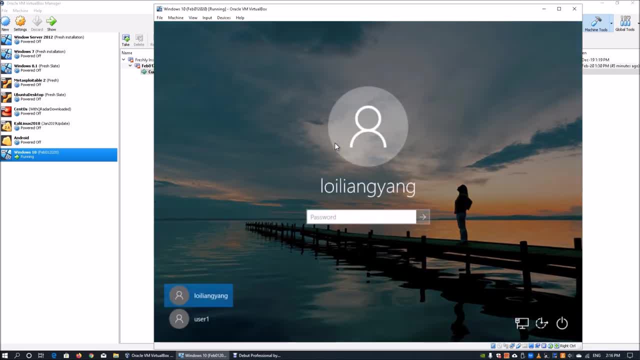 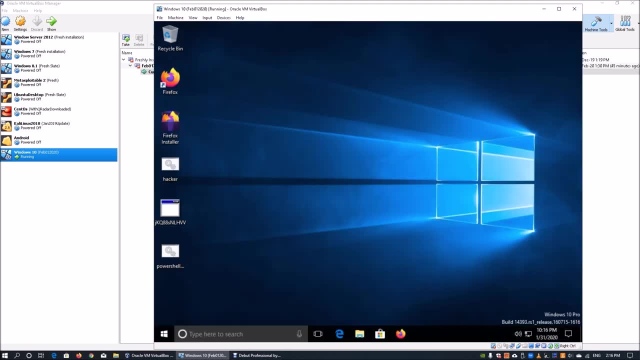 So over here I have Windows operating system running and we can go ahead and log in. So of course I got a username as loyliangyang and we can enter your password and we can access into the operating system. So, like I mentioned earlier, we are going to install.